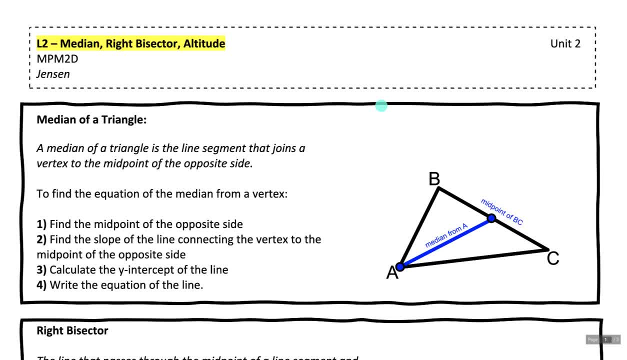 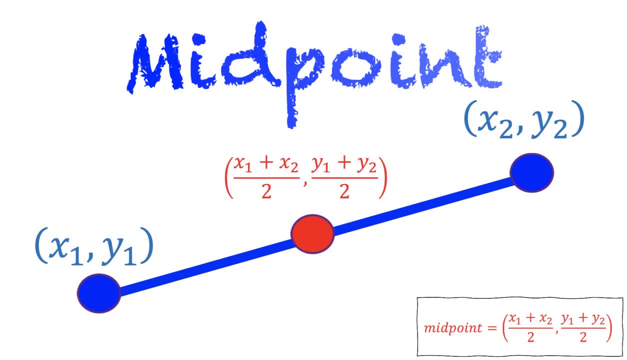 can complete this lesson is the midpoint formula. Notice, when finding the median of a triangle or the right bisector of a line, it involves the midpoint. And to find the midpoint of a triangle, we find the midpoint of a line segment. we find the average of the x coordinates of the end point. 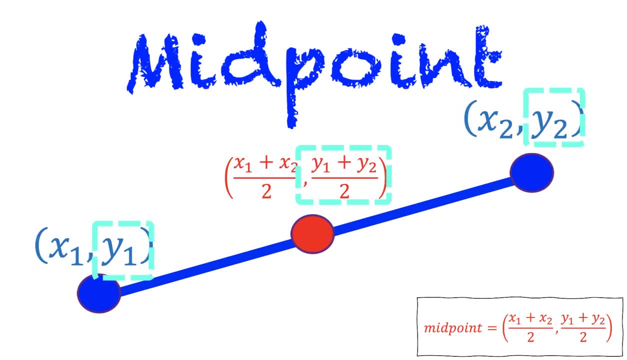 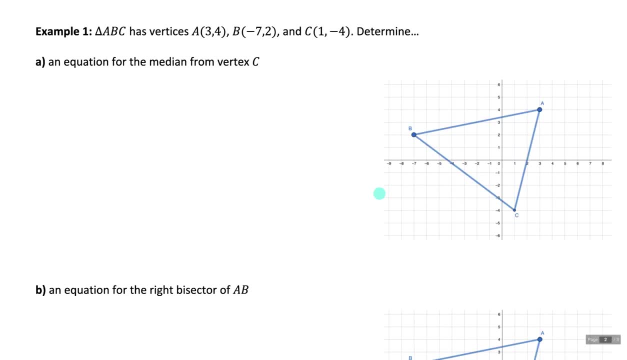 by adding them and dividing by 2, and then we find the average of the y coordinates of the end points by adding them and dividing by 2.. With all of that in mind, let's try our first example. Example 1 gives us triangle ABC. so we know the coordinates of all the vertices of the triangle and we need 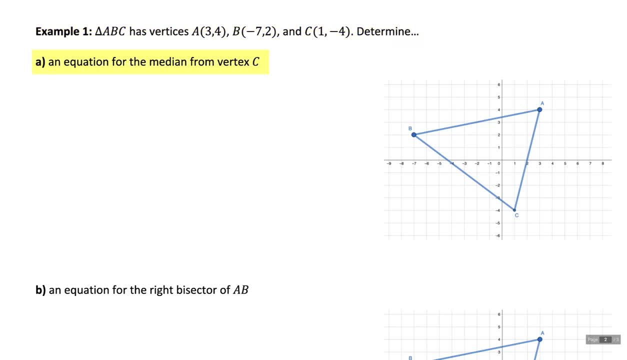 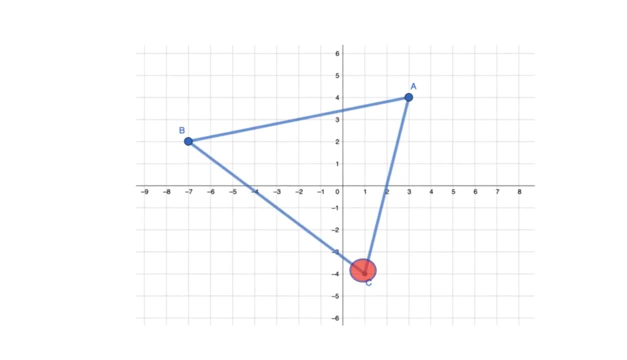 to, in part a, determine the equation for the median from vertex c, Based on the definition of a median. I know that the median of a triangle is the median of a triangle and I know that the median from vertex c will go from point c to the midpoint of the opposite side, So it'll go from c. 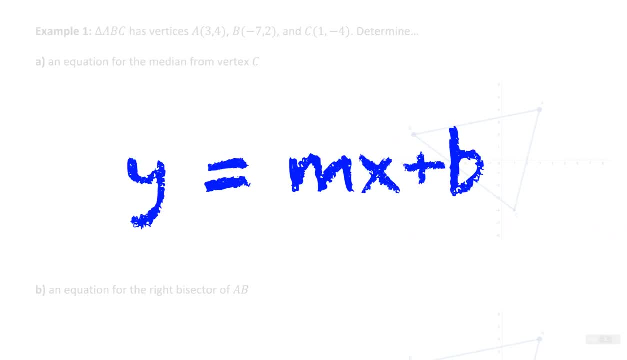 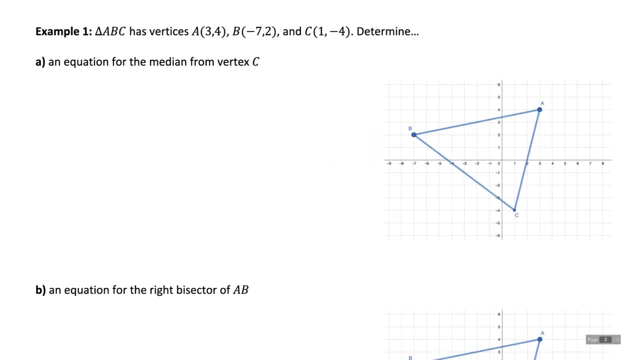 to the midpoint of ab. To find the equation of the median in the form y equals mx plus b, I will need to know the slope of the line and the y-intercept of the line. So let's think about how could we find the slope of the median? To find the slope of any line, you need to know two points on. 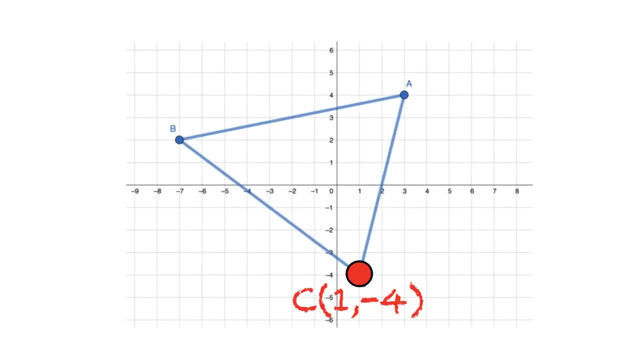 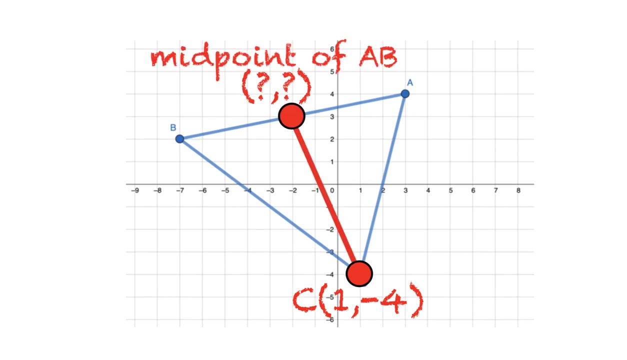 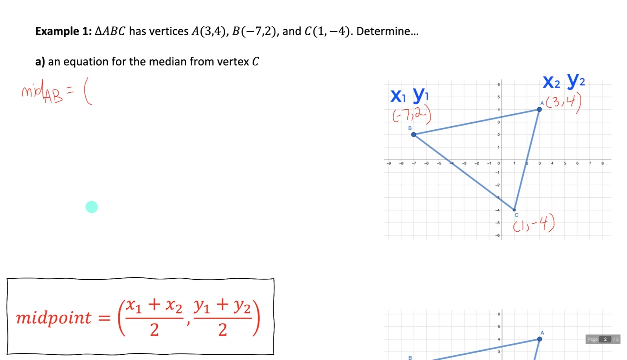 the line, While I know the median starts at c and I have the coordinates of vertex c and I know it goes to the midpoint of ab, So I'll need to calculate the coordinates of the midpoint of ab. To find the midpoint of ab I'm going to have to average the x-coordinates of. 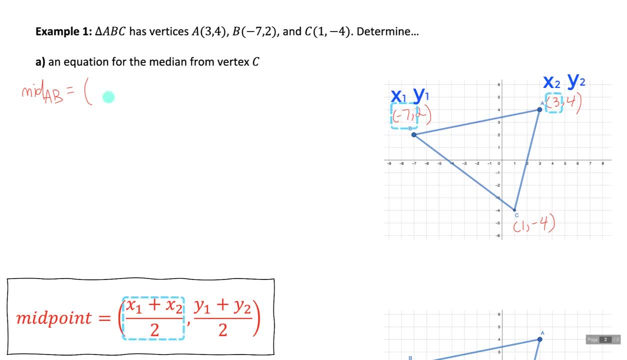 the endpoints. So to find the average of negative 7 and 3, I would add them and then divide by 2.. And I'll also have to find the average of the y-coordinates of the endpoints. So the average of 2 and 4, I can calculate by adding 2 and 4, and then dividing by 2.. So I'll need to know the 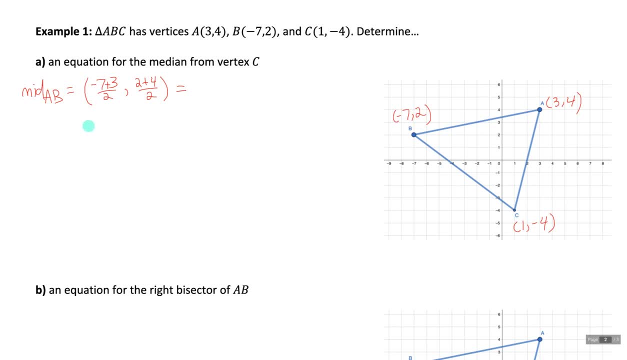 slope of the line and the y-intercept of the line. To find the slope of the line and the y-intercept of the line, I'll need to add them and then dividing by 2.. So my midpoint, the x-coordinate of the midpoint, will be negative 7 plus 3, which is negative 4, divided by 2.. So that would give 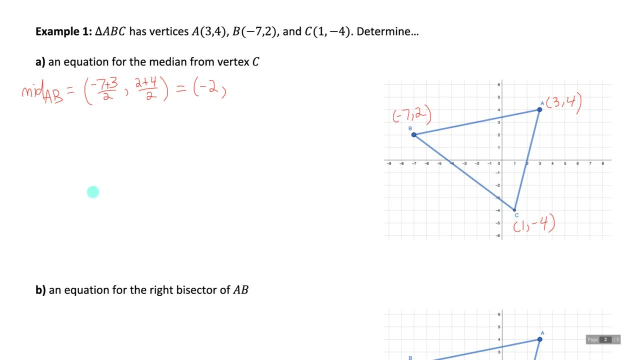 me negative 2.. And the y-coordinate of the midpoint, 2 plus 4, is 6, divided by 2 is 3.. So my midpoint is the point negative 2, 3.. Let me label that on the triangle and make sure it. 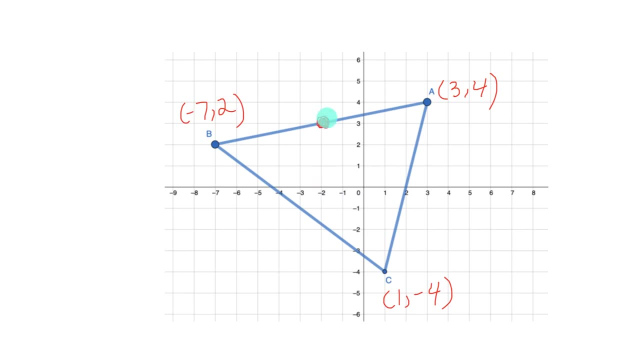 looks good. Negative 2,, 3,. that appears to be the midpoint. So there's my midpoint of ab. At this point I could draw the median That'll help me visualize it. It's going to go from c to the midpoint of the opposite side. So that's what the median looks like. 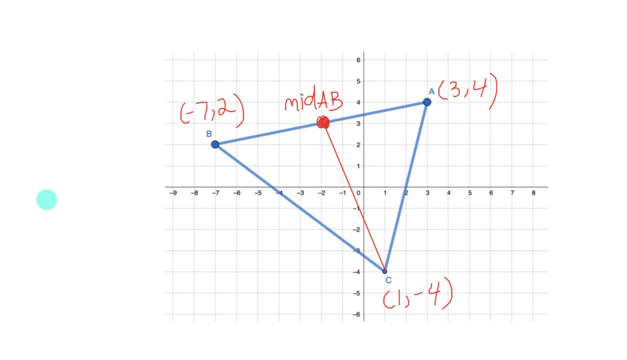 I'm going to determine the equation of that median in the form: y equals mx plus b. Now that I have the coordinates of the midpoint, I now have two points on my line. I have point c and the midpoint of ab. Those two points are both on the median, so I can now calculate the slope of the median. 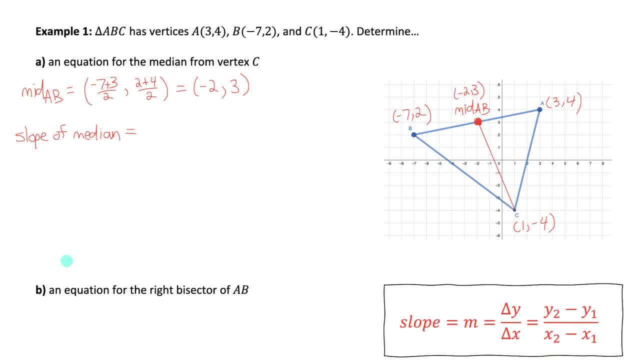 by calculating the change in y over change in x. So I'll use the formula y2 minus b, y1 over x2 minus x1.. I'll choose point c to be my second point. It doesn't have to be, It could. 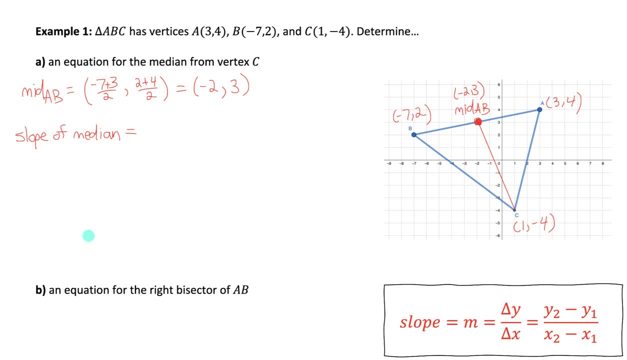 be my first point, but I'll choose it to be my second And I'll do y2 minus y1, so negative 4 minus 3, divided by x2 minus x1, 1 minus negative 2. This calculation will give me negative 7. 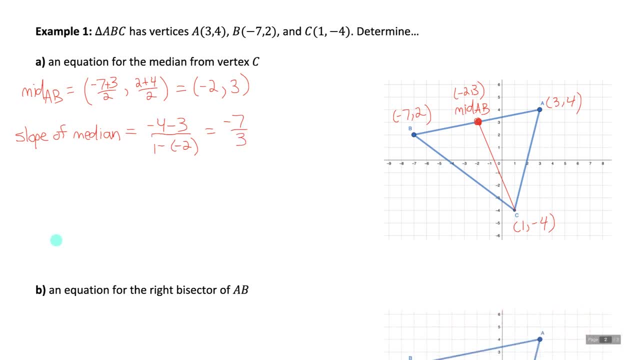 over 3.. That's the slope of my median. Remember to write the equation of the median. I'm going to be writing it in the form: y equals mx plus b. So I'm going to write it in the form: y equals mx plus b. I now have my m, but I don't know the value of b. To calculate the value of b. 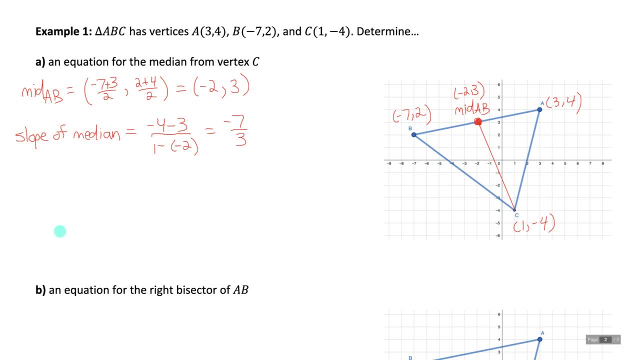 I'll sub in negative 7 over 3 for m and any point xy that is on my line. I have two points that are on the line. I can choose either c or the midpoint of ab to be my xy. I'll choose point c, So let me. 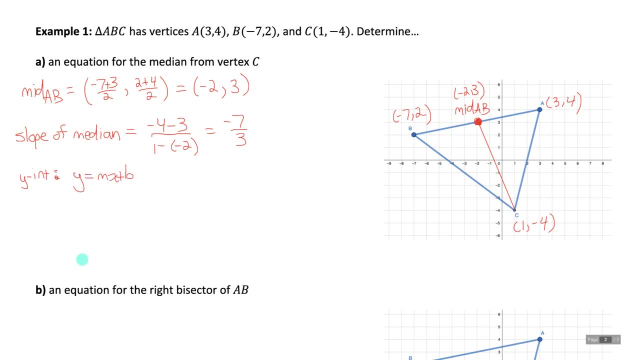 solve for the b value, which is the y-intercept Into y equals mx plus b. I can sub in the point c. So negative 4 equals and m, I know, is negative 7 over 3.. x is 1.. The only value I don't know is b. 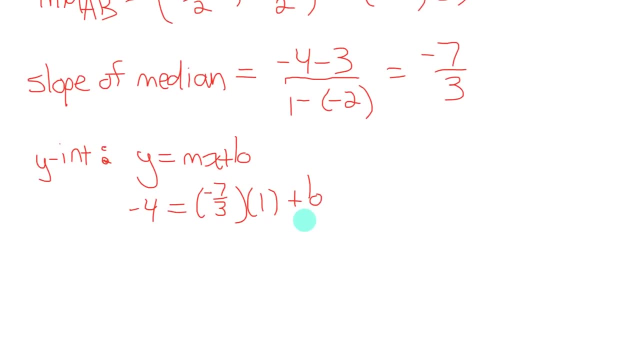 And then we just have to rearrange this and solve for b. So I'm going to want to isolate b. So I'm going to take this negative 7 over 3 times 1, that's just negative 7 over 3,. 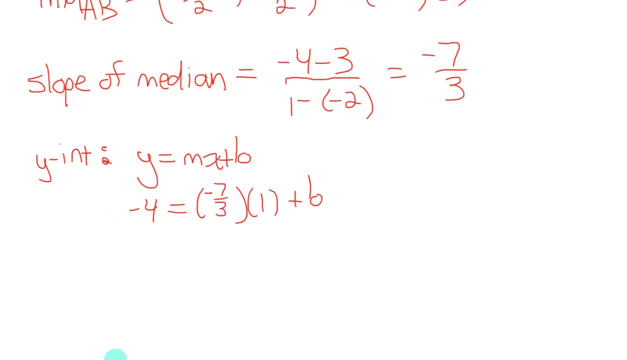 and move it to the left. It's going to be added to negative 4, and I'm going to want a common denominator, So I'm going to rewrite negative 4 as negative 7 over 3.. Negative 12 over 3, right. Negative 12 divided by 3 is negative 4.. It's just rewriting it in an 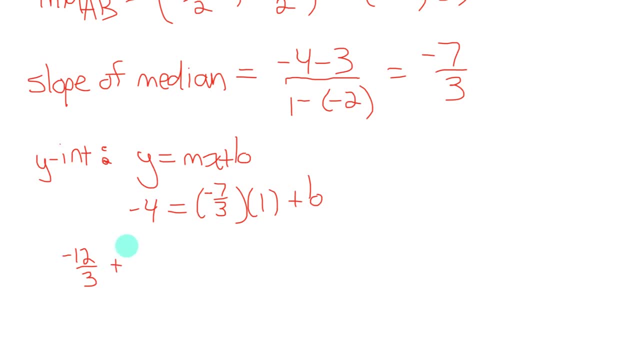 equivalent form that has the same denominator as 7 over 3, so that I can collect them together: Negative 12 over 3 plus 7 over 3 is negative 5 over 3.. So my b value is negative 5 over 3.. 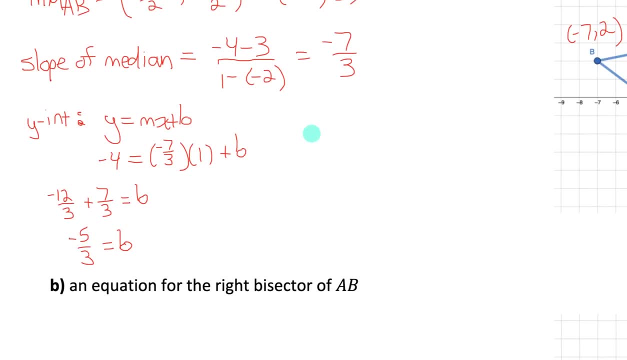 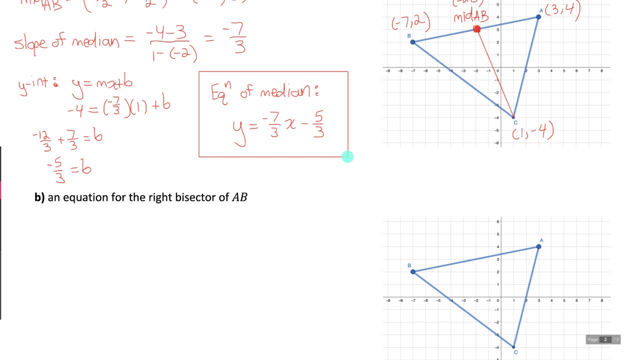 With all of this I can write my final answer: the equation of the median. So the equation of the median is: y equals negative 7 over 3x minus 5 over 3.. Now that line y equals negative 7 over 3x minus 5. 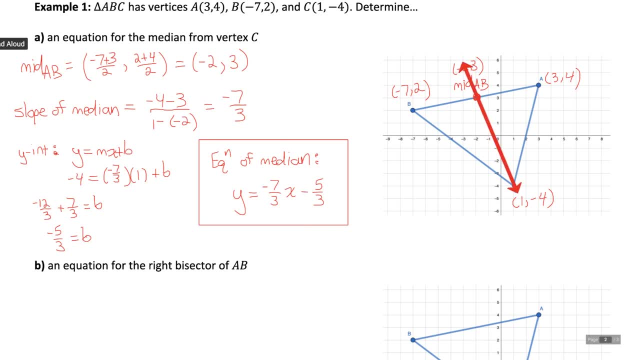 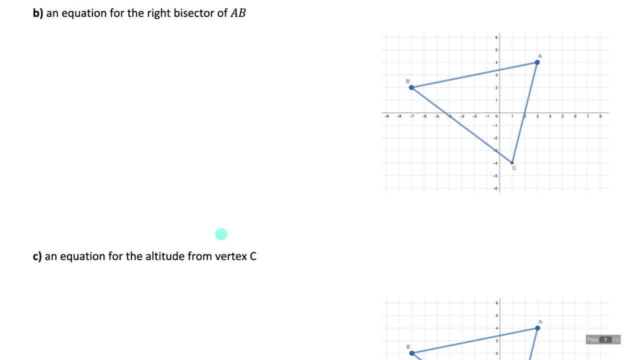 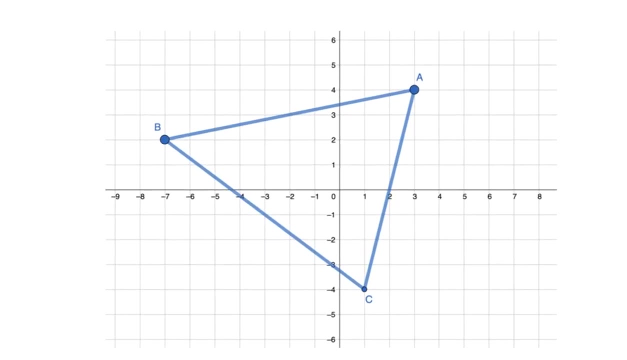 over 3, is a continuous line that would go forever, but the median of this triangle falls on that line and is contained within the triangle. Let's now do a right bisector question. So part b asks us to find an equation for the right bisector of ab. If you remember, a right bisector is a line that is. 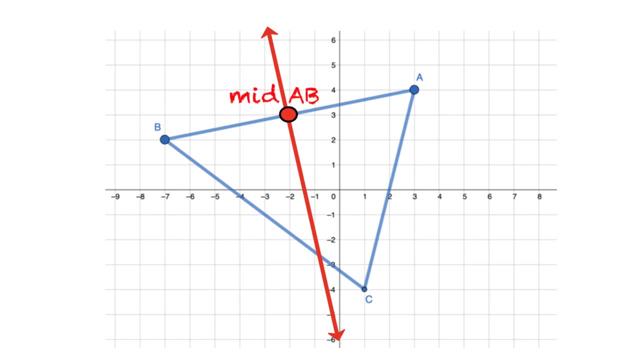 going to intersect line ab at its midpoint And it is going to intersect it at a 90 degree angle. In the previous question we calculated the midpoint of ab to be the point negative 2, 3.. We already have that. So I know an xy point on my right bisector To find the slope of the right bisector. 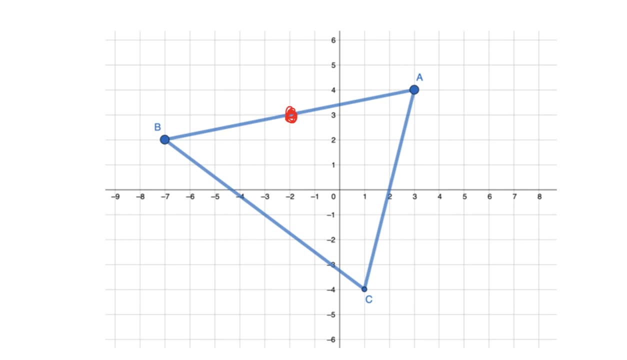 we're going to have to do it a little bit differently, Since we only know a single point on a right bisector. we're going to have to use the fact that it's perpendicular to ab to be able to calculate its slope. So let me start by figuring out what is the slope of ab. 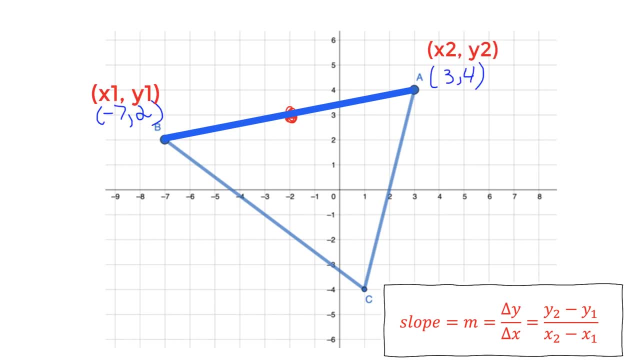 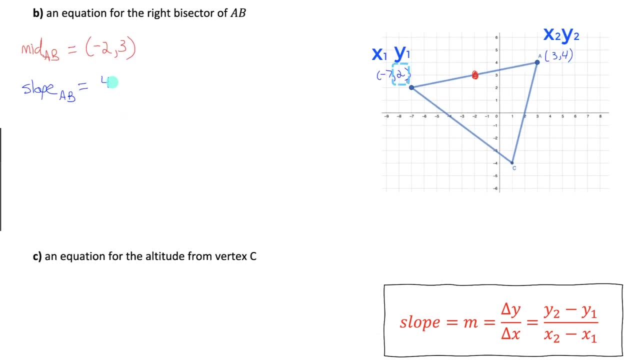 So let's calculate the slope of ab. To calculate the slope of ab I'll have to find change in y over change in x. so I'll find the difference in the y coordinate 4 minus 2, divided by the difference in the x coordinates 3 minus negative 7.. And that gives me 2 over 10,. 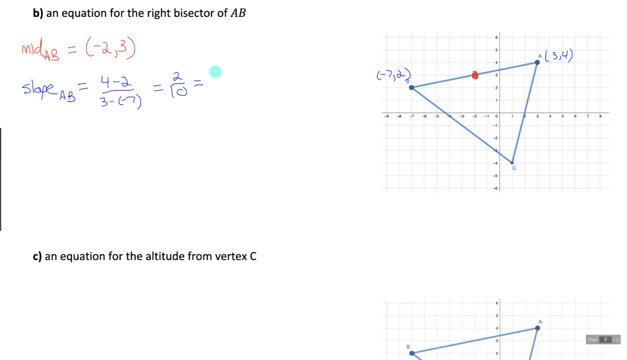 which I could reduce 2 into both 2 and 10, it foes into 2 along with 10. five times The slope of line ab is 1 over 5. And you can see to get SO I want you to ask these Things to radiate between their RAW field and ground suggestion. 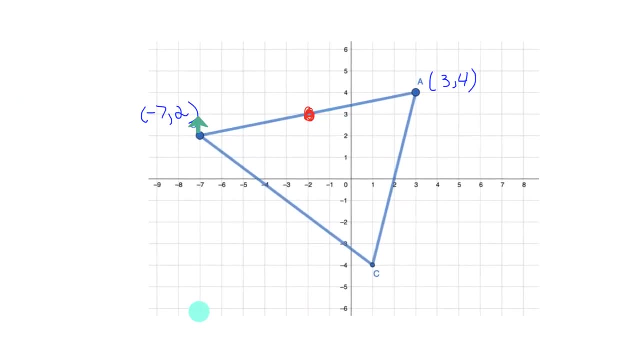 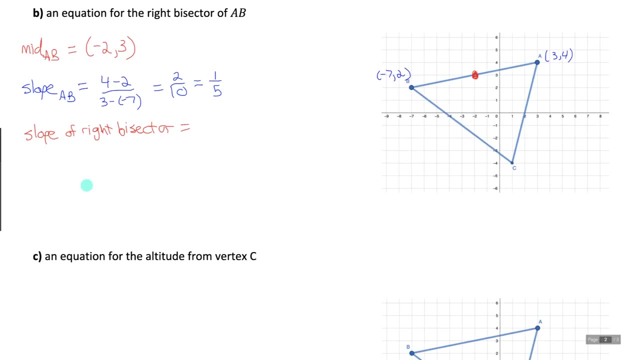 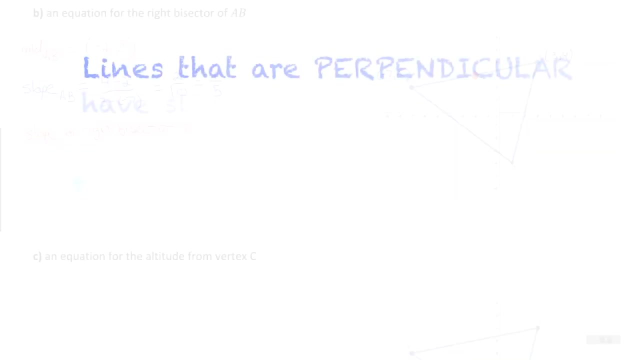 point b to the midpoint of the line, you rise one and run five, so that that looks like the correct slope of line segment a b. now that i know the slope of line a b, i can find the slope of the right bisector by using the principle that tells me that lines that are perpendicular to each other. 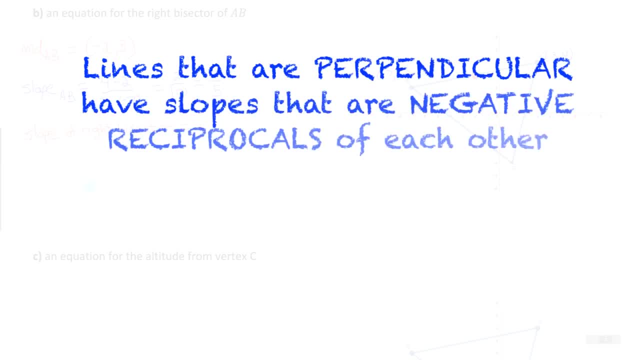 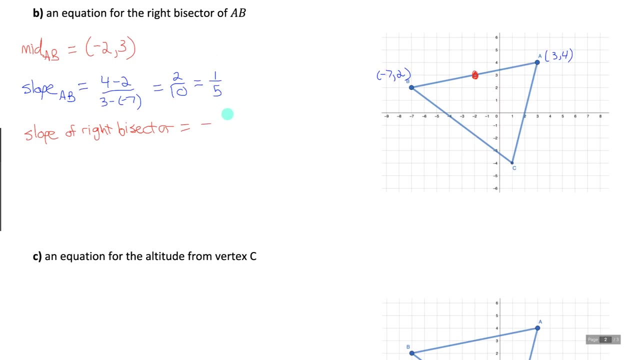 have slopes that are negative reciprocals. to calculate a negative reciprocal slope, we multiply it by negative one, which effectively changes its sign, and then we find the reciprocal of it, which means flip it. so instead of positive one over five, it changes to negative five over one. 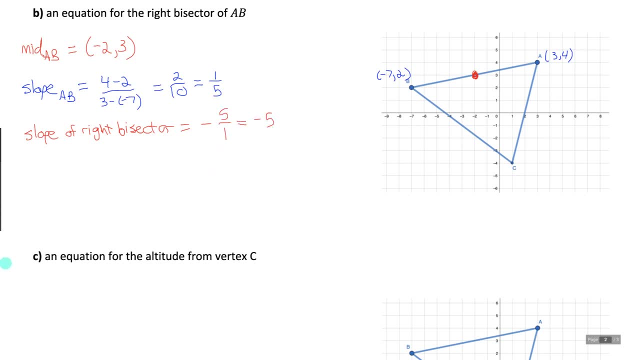 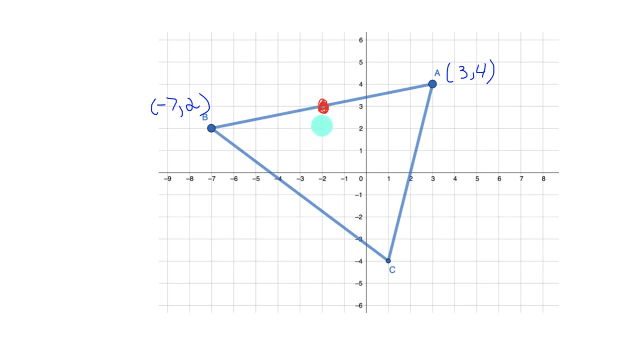 and negative five divided by one is just negative five. so the slope of my right bisector is negative five. so if i wanted to, i could accurately draw the right bisector now by from the midpoint of a, b. i could use the slope negative five over one. that means down five. one, two, three, four, five. 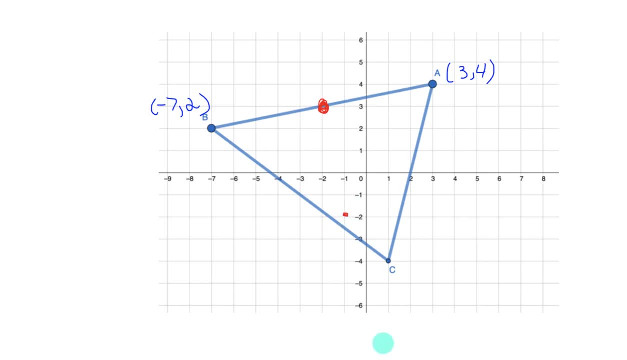 over one and plot a point. now that i see two points on the line, i can draw a line through those two points and that would be my right bisector. so that's the right bisector of line segment a- b. let me just put a little right angle symbol here to show you that it forms a 90 degree angle with line segment a- b. 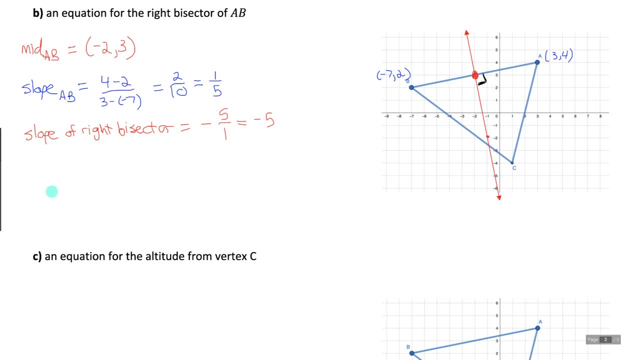 so that's what it looks like, but what's its equation? we know the slope. we know m is negative five. we don't yet know b, the y-intercept. i can solve for the y-intercept by into the equation plus b, subbing my slope of negative five in for m and plugging in any point that is on my right. 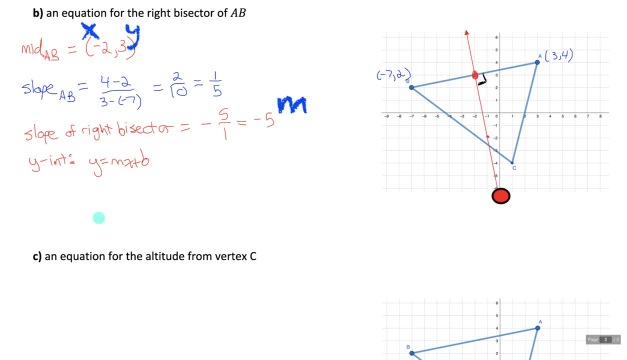 bisector in for x and y. the one point i know for sure, that is on my right bisector is the midpoint of a, b, the point negative two, three. so i'll plug three in. for y, the slope of my right bisector is negative five and the x coordinate of the midpoint was negative two. if i solve this for b, negative five. 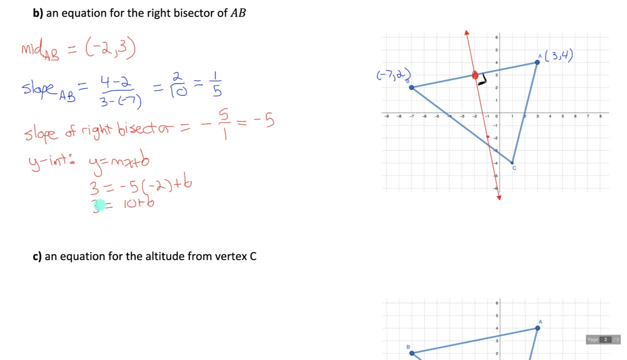 times negative. two is ten. subtract the ten to the other side, three minus ten is b. therefore b is negative seven. now that i have all of that information, i can write the equation of the right bisector. the equation will be: y equals negative five x minus seven. part c asks us to find the equation. 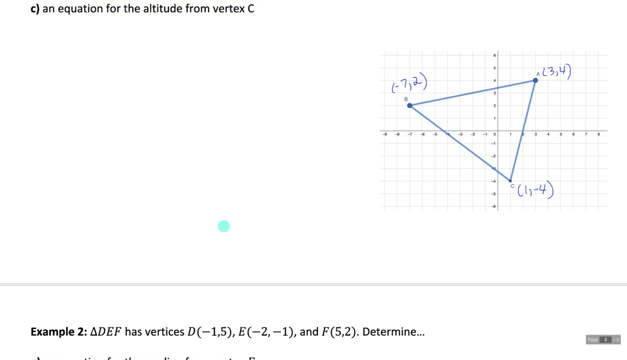 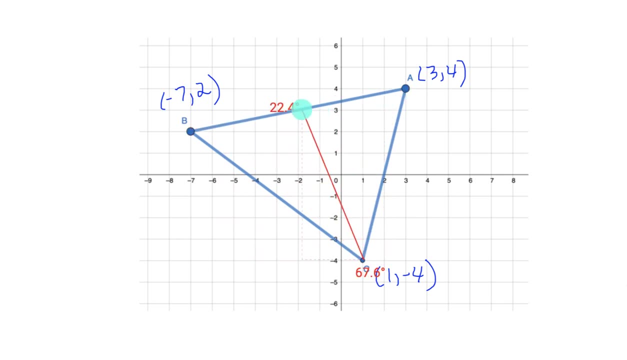 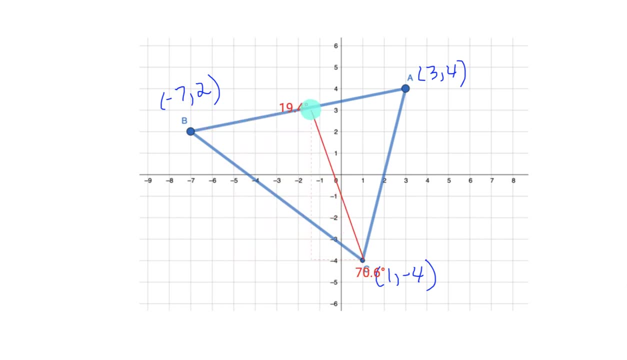 so it's not necessarily going to go to the midpoint. it's going to go to whatever point makes it form a 90 degree angle with the opposite side. so we'll have to do some calculating to figure out in what direction the altitude is actually going to go, since i know it's going to make a 90 degree angle. 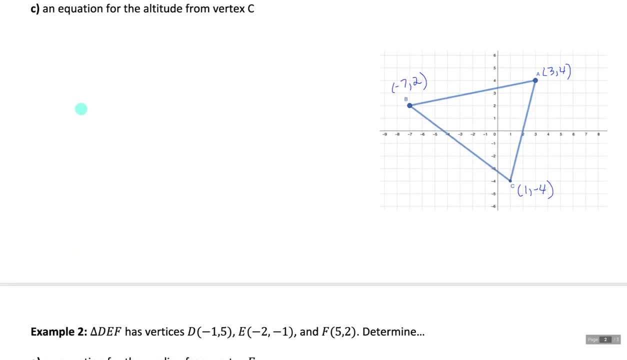 with the opposite side. i know it's going to have a slope that is perpendicular to the opposite side and, if you remember, we've already calculated the slope of a- b. the slope of a- b: when we did the change in y over the change in x, we got 2 over 10, which is 1 over 5.. that would mean that the 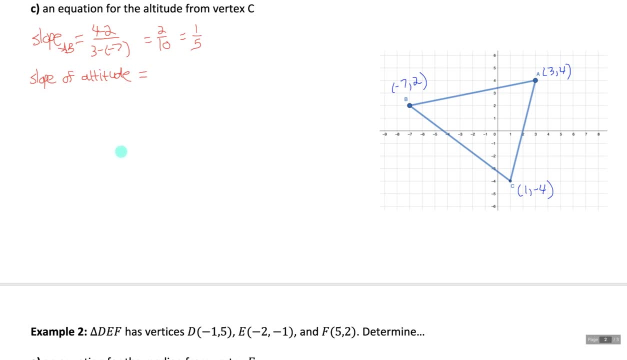 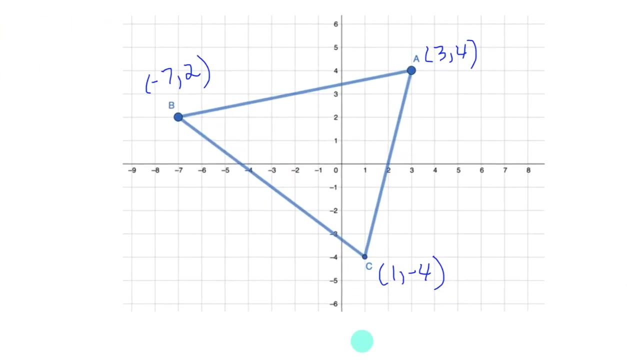 slope of the altitude is the negative reciprocal of that. that means flip it and change the sign. so instead of positive 1 over 5 it becomes negative 5 over 1.. so knowing that slope i could do an accurate sketch of the altitude. a slope of negative 5 over 1 means down five right. 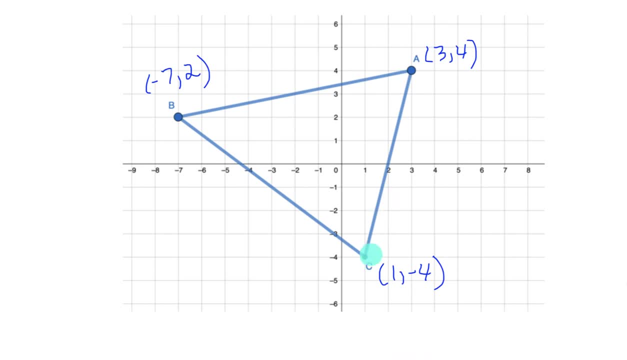 one, but that'll give me a point outside the triangle. so i'll do the opposite: up five, one, two, three, four, five, left one. so i now know the direction of this altitude. i can connect those points and go all the way to the opposite side, and there's my altitude to write the equation of that. 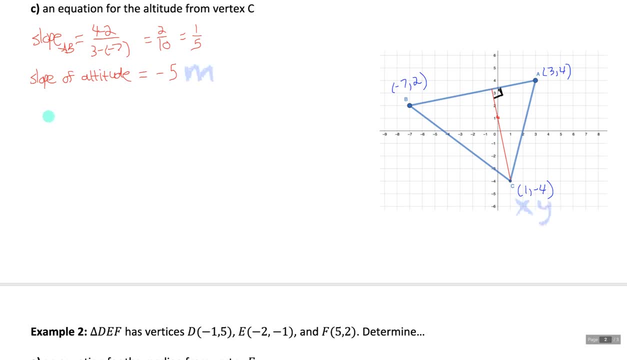 altitude in the form y equals mxp plus b. i know m it's negative five, but i'll have to solve for b the y intercept, and i can solve for that by subbing into y equals mx plus b the slope of negative five for m and any xy point. 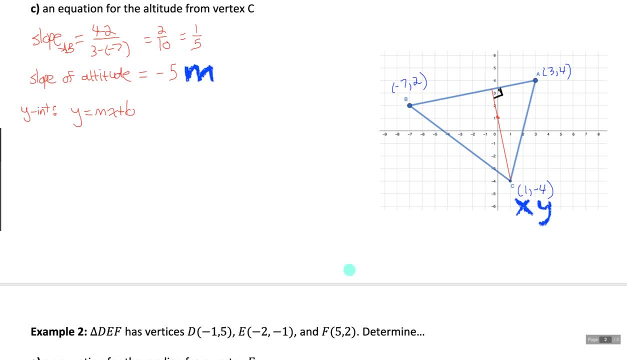 that is on the altitude, and the only point that i know is on the altitude is point c. so i'll use one for x and negative four for y. so negative four equals negative five times one plus b. negative four equals negative five plus b. add the five to the other side. 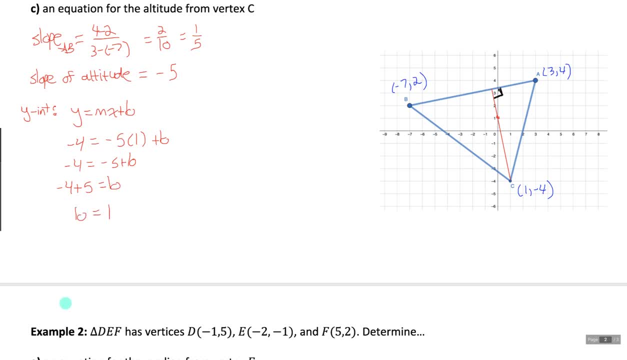 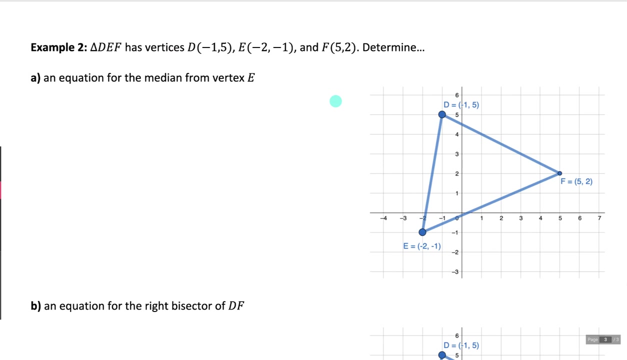 and i figure out that b is one, so i can write the equation of the line that the altitude falls on. y equals negative five x plus one. let's do another example. i'll go through them more quickly this time. but we're going to do another: median, right, bisector and altitude of this triangle, triangle def. so the first thing we're 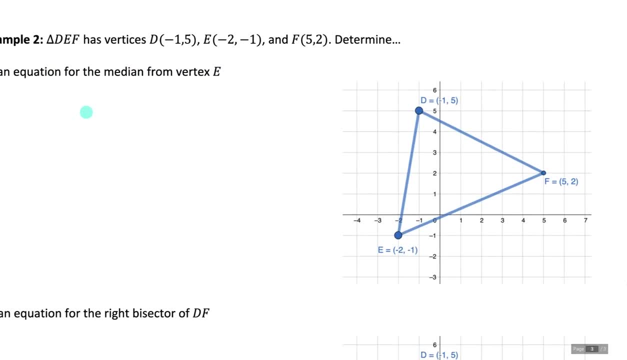 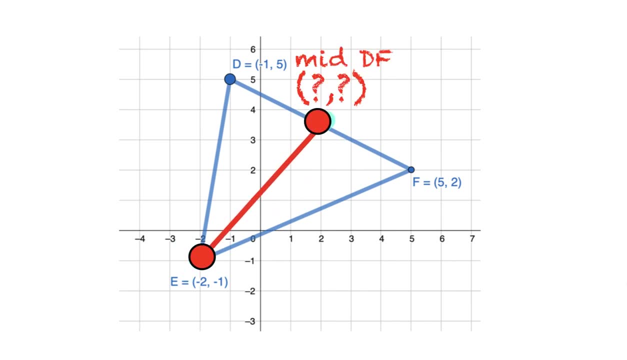 going to find is the median from vertex e. if i want the median from e, i know, based on the definition of median, it's going to go from e to whatever the midpoint of the opposite side is. so i'll have to start by calculating what is the midpoint of the opposite side? 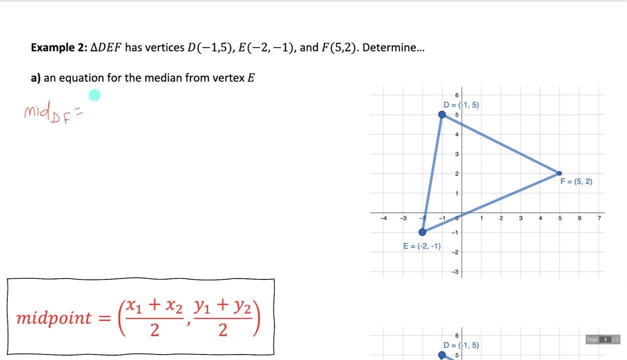 so the midpoint of df can be calculated by finding the average of the x-coordinates of the endpoints. and i can average negative one and five by adding them and dividing by five, 2. And I'll also find the average of the y-coordinates of the endpoints. So I'll find the average. 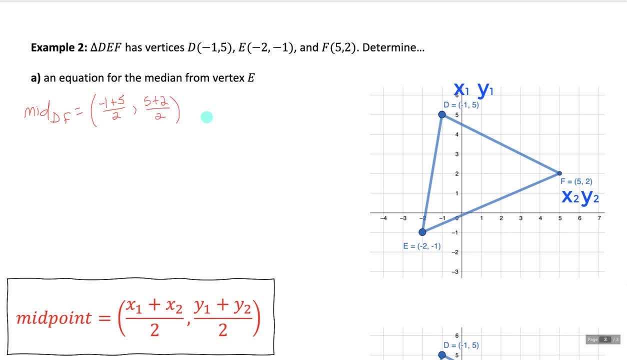 of 5 and 2 by adding them and dividing by 2.. The x-coordinate of the midpoint negative, 1 plus 5, is 4,, divided by 2 is 2.. And the y-coordinate 5 plus 2 is 7, over 2.. So 7. 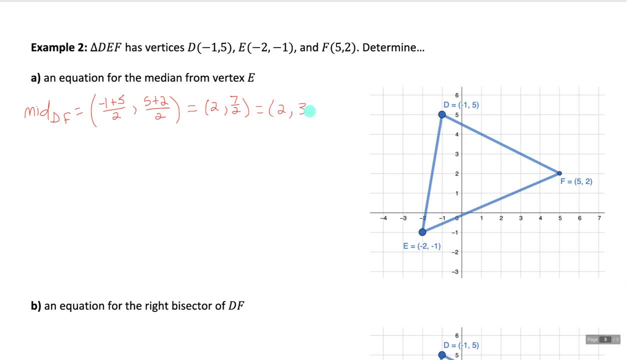 over 2.. If you wanted to write that as a decimal, it would be 2, 3.5.. So that would be this point, right here. That's the midpoint of df, So I can now draw the median. It's the. 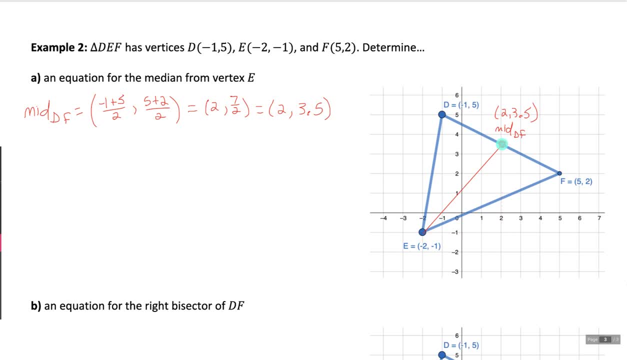 line that's going to go from e to the midpoint of the opposite side. To write the equation of that line in the form y equals mx plus b, I need to know the slope of the line and the y-intercept of the line. I can find the slope of the line by using the formula y2. 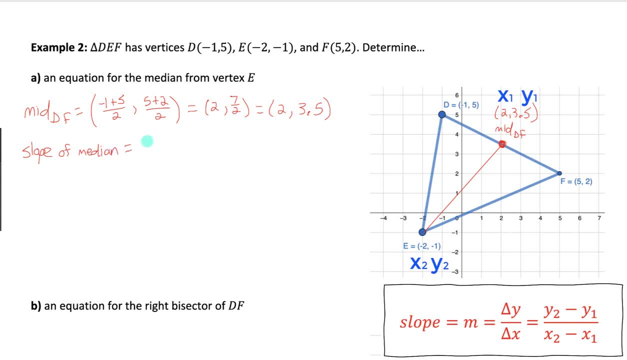 minus y1 over x2 minus x1.. So I'll find the difference in the y-coordinates. I'll do 3.5 minus y2 minus y1.. 2 minus negative 1 over the difference in the x-coordinates 2 minus negative 2.. So 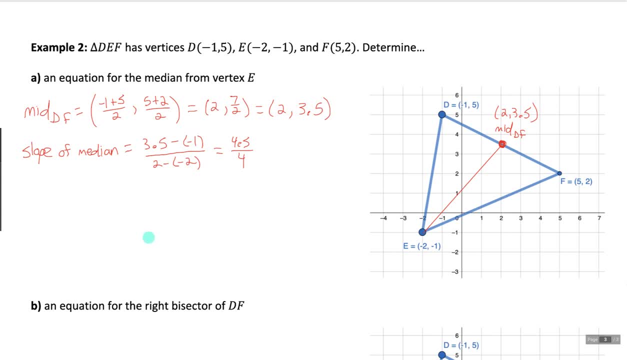 that gives me 4.5 over 4.. And if I were to write that with integer values and get rid of the decimals, I can multiply top and bottom of that by 2, and that would give me 9 over 8.. So my m value, my slope, is 9 over 8.. And I could have got that same answer by instead. 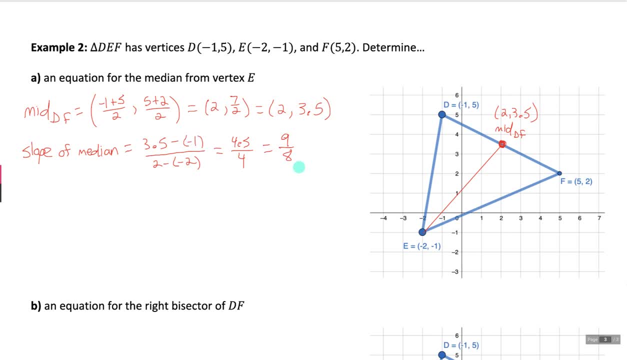 of using 3.5, I could have used the fraction 7 over 2.. Let me show you what that would look like. So I would do 7 over 2, minus negative 1.. But I would want a common denominator, so I would. 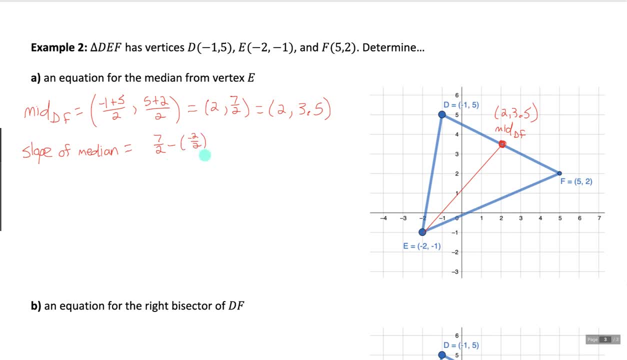 write negative 1 as negative 2 over 2. That's equivalent to negative 1. Over the change in x, which would be 2 minus negative 2.. So in the numerator I've got two fractions being subtracted that have a common denominator, So I could just subtract their numerator. 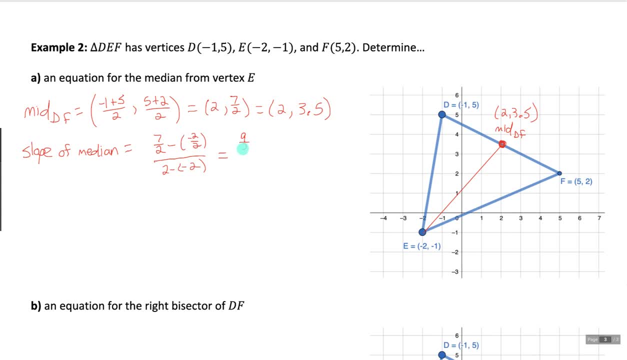 7 minus negative 2.. That's 9.. Keep the denominator, so 9 over 2.. Over 2 minus negative 2 is 4.. I could think of that as 4 over 1, if that helps. When dividing fractions you keep the. 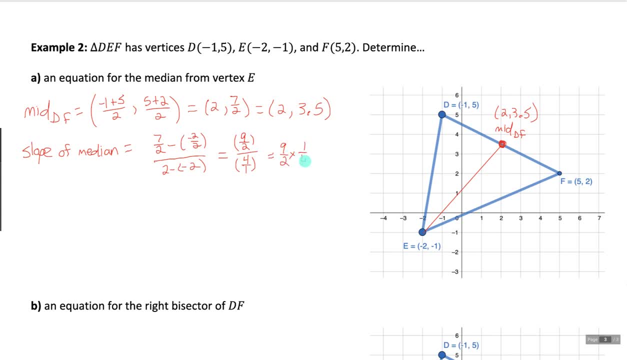 fraction in the numerator and multiply it by the reciprocal of the denominator. that gives me: 9 times 1 is 9, over 2 times 4 is 8.. So that's just another way of getting the same answer that we had. Now that we know the slope, the m value, I can calculate the. 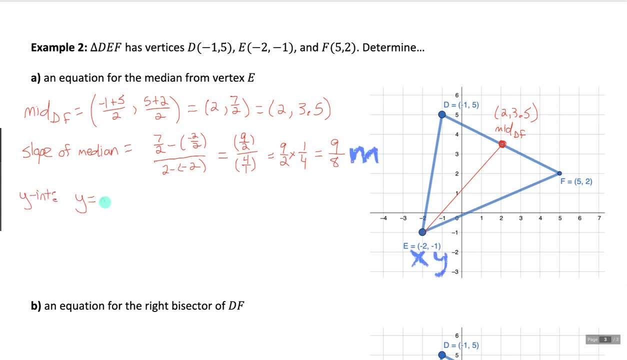 y-intercept. the b value by subbing into y equals mx plus b. my m value of 9 over 8, and any point on my median median for x and y. I'll choose point E for my median, since that one doesn't have any. 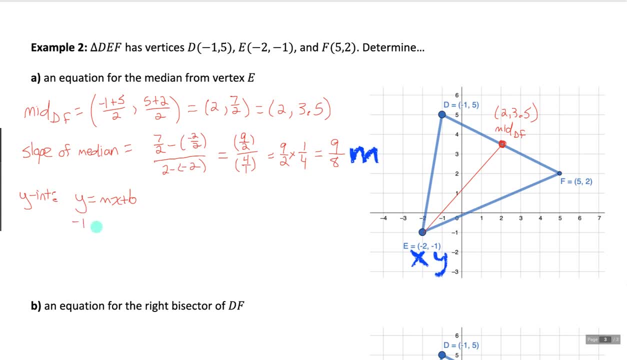 fractions. So point E, the y value is negative 1,, my slope is 9 over 8, and my x value is negative 2.. My only unknown here is b. I can solve for b. I'm actually going to reduce. 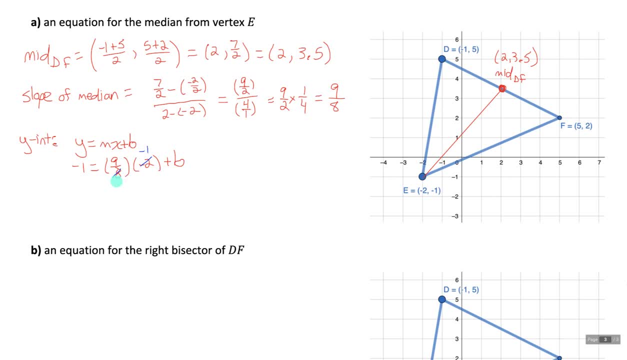 negative 2 over 8 to negative 1 over 4.. So I have 9 over 4 times negative 1, that's negative 9 over 4.. When I bring that to the other side it becomes positive 9 over 4. And I'm 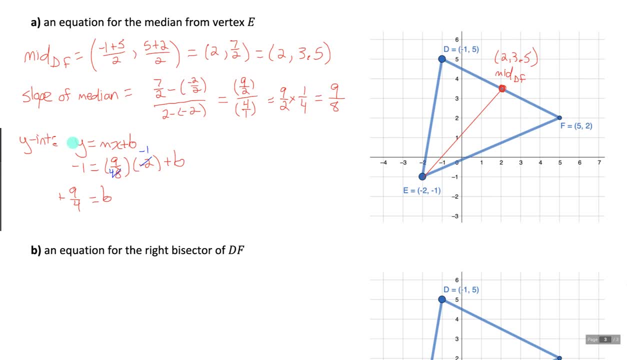 going to want to add it to negative 1, so I'm going to rewrite negative 1 with a denominator of 4 by writing it as negative 4 over 4.. So that gives me a b value of 5 over 4.. So I 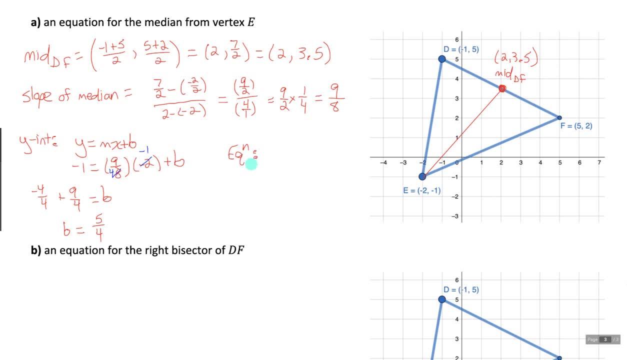 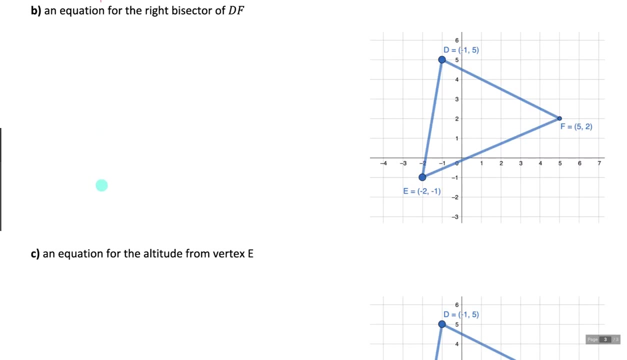 can now write the equation of the line that the median falls on and that equation would be: y equals 9 over 8x plus 5 over 4.. Let's now do the right bisector of df. The right bisector of df, I know will pass through. 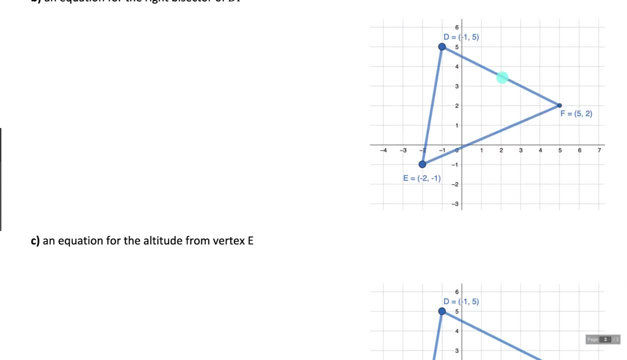 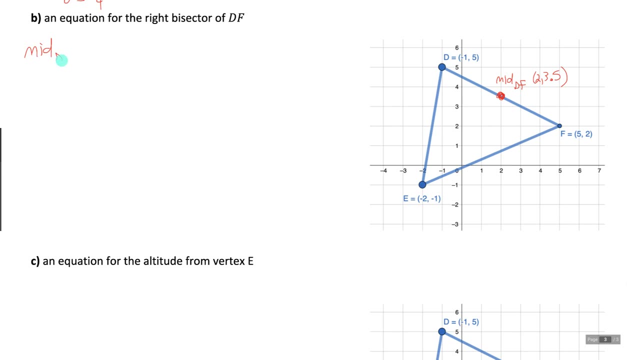 the midpoint of df, which we've already calculated as the point 2, 3.5, so I'm going to label that, And I know it's going to intersect df at a 90 degree angle, So I'll just record that here as well. mid df is 2, 7 over 2, or as a decimal, 2, 3.5.. And I know it's going. 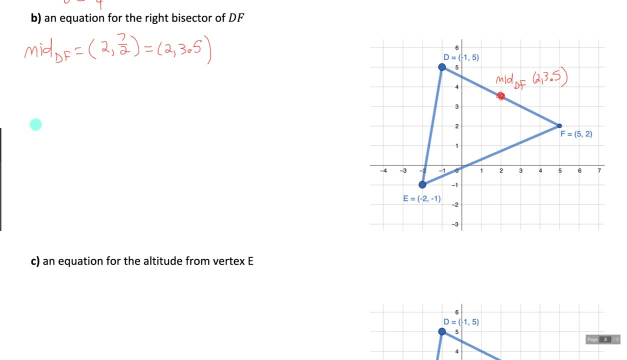 to intersect df at a 90 degree angle. So now we need to know the slope of df and then use its negative reciprocal as the slope of my right bisector. So let's find the slope of df by using my slope formula, y2 minus. 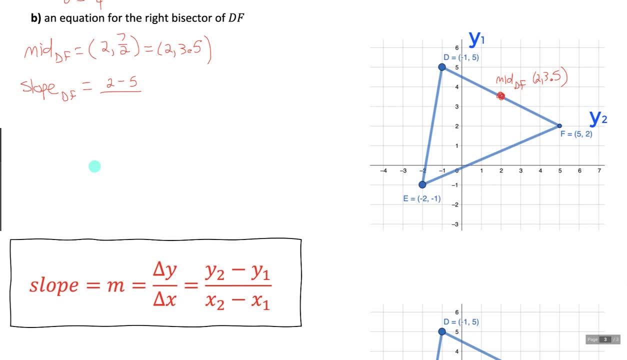 y1 over x2 minus x1.. So I will do 2 minus 5 over 5, minus negative 1, which gives me negative 3 over 6, which reduces to negative 1 over 2.. If that's the slope of df, I know my right bisector is perpendicular to that. so the 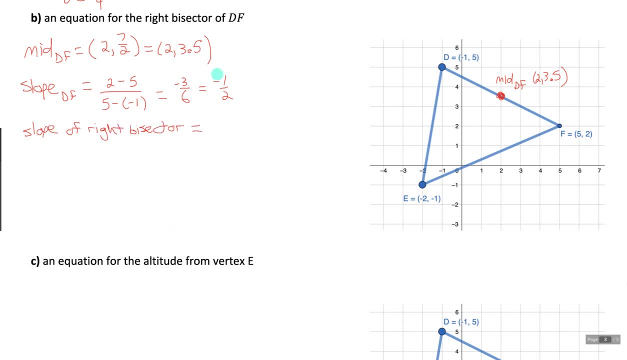 slope of my right bisector is going to be the negative reciprocal of negative one over two. So I need to change its sign. so it's going to become positive and use the reciprocal, which means flip it. So, instead of negative one over two. 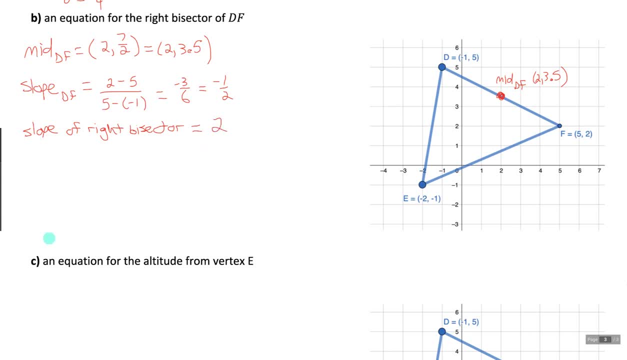 it's going to be positive two over one, which I can just write as positive two. Now that I know the slope, all I need to be able to write the equation is the y-intercept, the b value. So into y equals mx plus b. 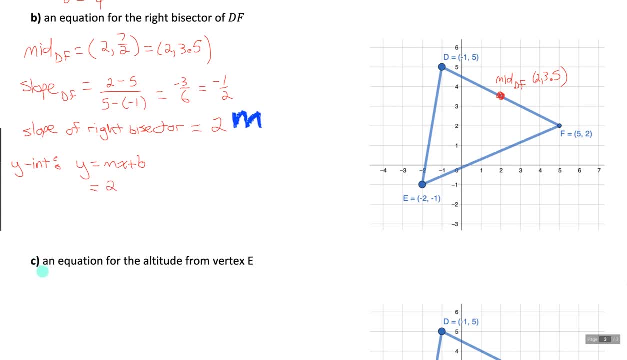 I know the slope is two, and then for x and y, I sub in the x and y coordinates of any point on my right bisector. The only point that I know is on my right bisector is the point two, 3.5.. 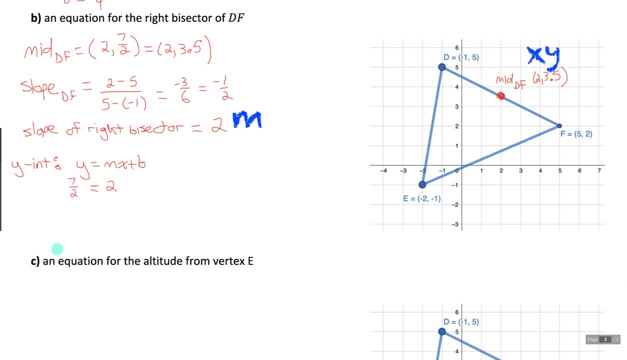 So I'll plug in 3.5 for y, I'll write it as a fraction: seven over two and two for x. Now I can solve for b. So I've got seven over two equals two times two is four plus b. 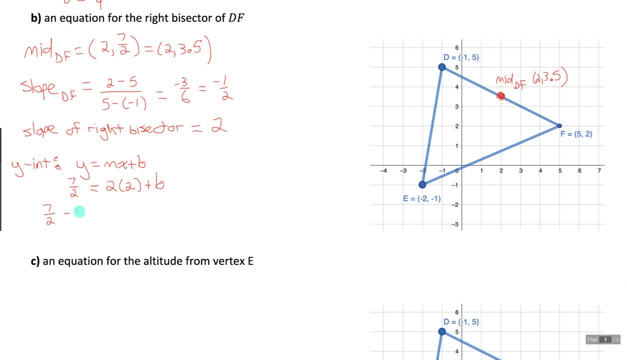 So I'll move that four to the other side, so it'll be minus four. I'm going to want to collect it with seven over two, so it's going to need to have to have a common denominator. So right now it's a four over one. 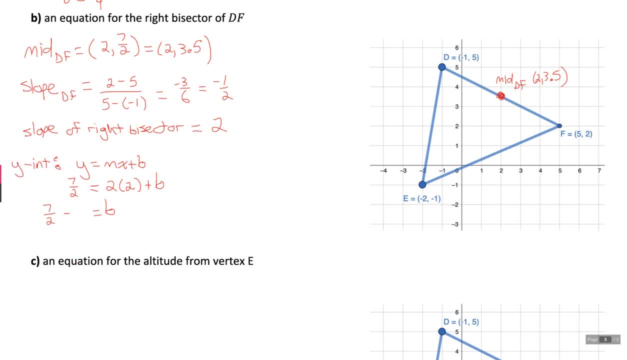 I'll have to multiply top and bottom by two and that will give me eight over two, which is equivalent to four. So I have seven over two minus eight over two. That gives me a b value of negative one over two. So my equation of my right bisector. 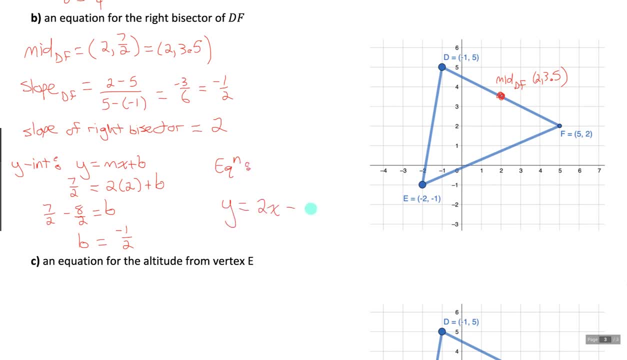 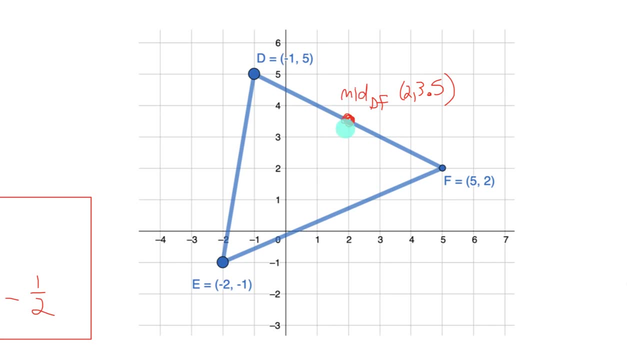 is going to be: y equals two x minus a half. Let me actually draw that right here, So I know it goes through this midpoint here, this point two, 3.5.. From there I can use the slope of two, which we can think of as two over one. 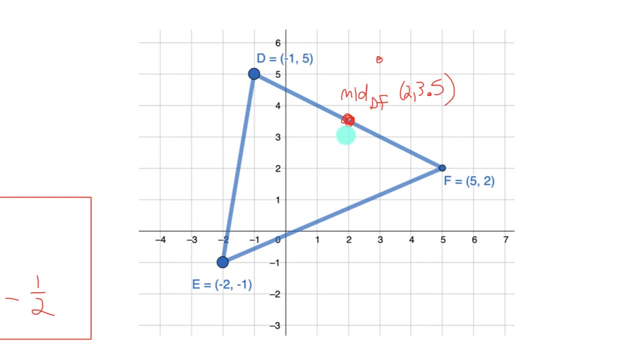 to go up to right one or down to left one. I'll plot another point just so we can see. So, down one, two, left one. That's going to cross the y-axis where we said it would. It's going to cross at negative a half. 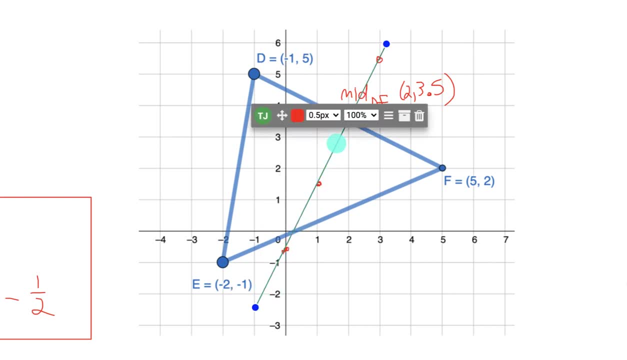 And let me connect these points And I'll put arrows on the ends of this line to show it's a continuous line. There's my right bisector. Notice it goes through the midpoint of df and it intersects it at a 90 degree angle. 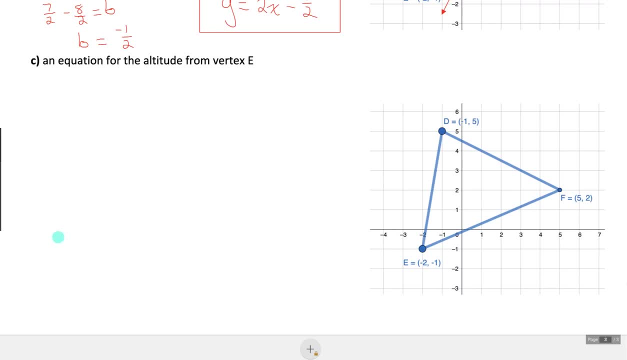 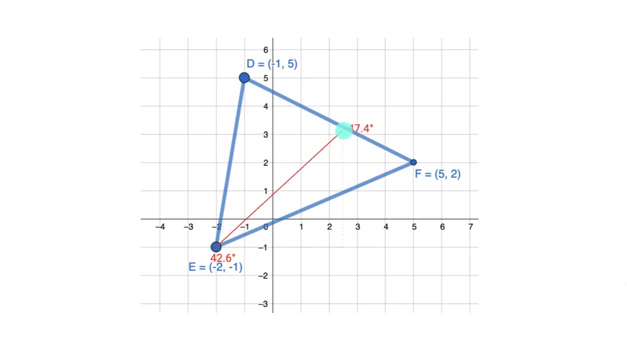 Last part of the lesson we'll find the altitude from vertex e. I know an altitude is going to go from the vertex of a triangle to the opposite side at a point where it's going to make a 90 degree angle at the opposite side. 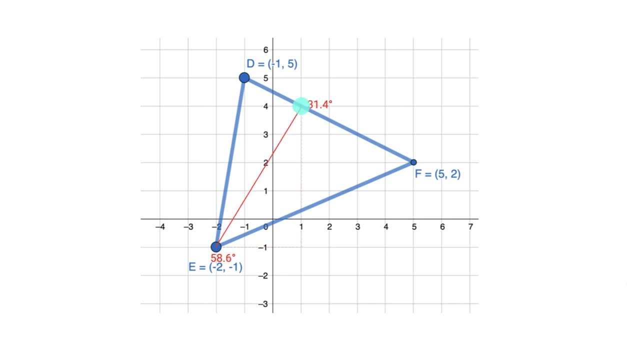 So it's not going to go to the midpoint, It's going to go somewhere else so that when it connects it forms a 90 degree. It looks like it's going to be around here. So the fact that I know that it's going to be- 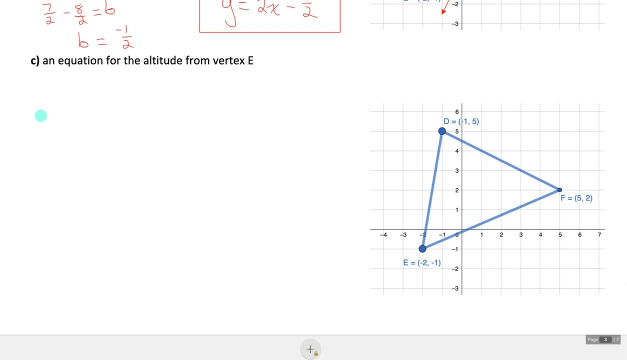 perpendicular to df tells me that I'll be able to find the slope of it by using the negative reciprocal of the slope of df. And if you remember from the last question, we know the slope of df is negative one over two. That tells me the slope of my altitude. 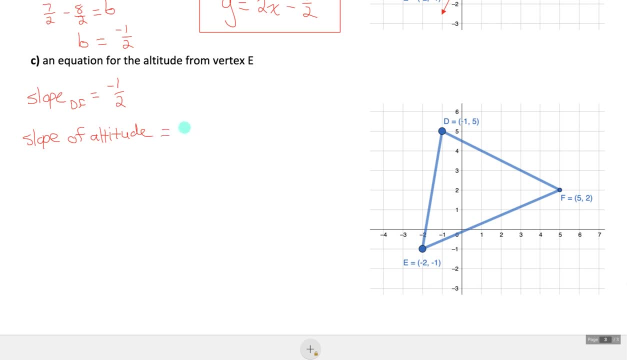 is going to be the negative reciprocal of that. So it's going to be positive two over one, which I'll write as positive two. So I know from e it's going to go up two right one. Up two, right one. 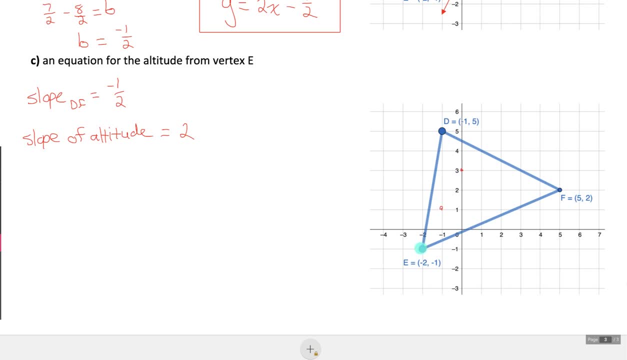 And so on, Until it connects to the opposite side. So this is what the altitude's going to look like. Based on how I drew it, it looks like the y-intercept is going to be three, or at least about three. Let's do some calculating to make sure.